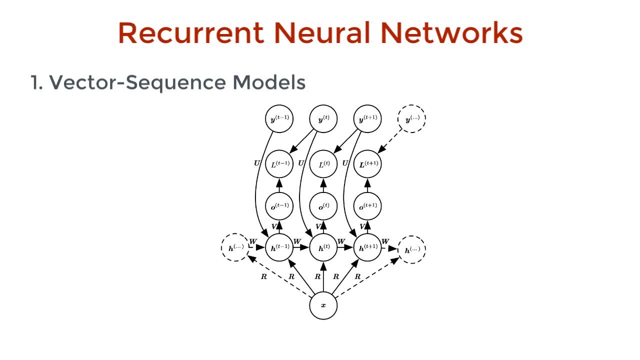 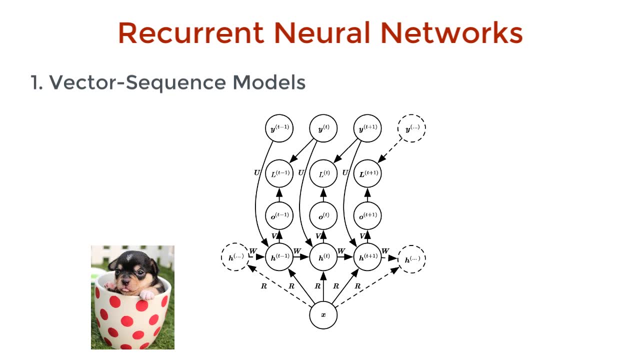 These neural nets take in a fixed-size vector as input and it outputs a sequence of any length. In image captioning, for example, the input can be a vector representation of an image and the output sequence is a sentence that describes the image. 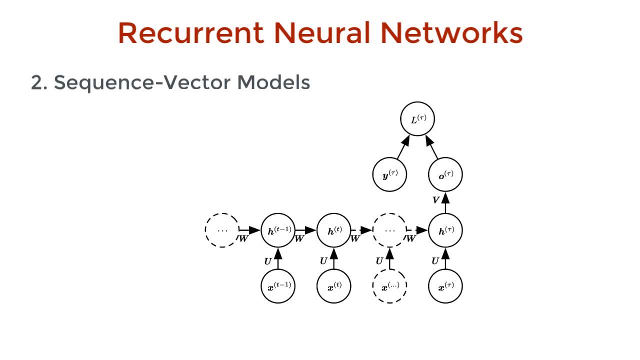 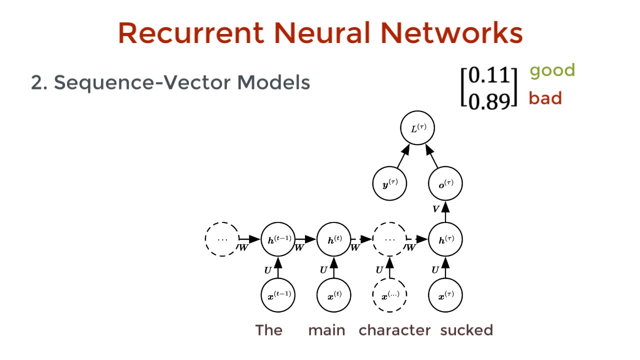 The second type is a sequence-to-vector model. These neural networks take in a sequence as input and spits out a fixed-length vector. In sentiment analysis, the movie review is an input and a fixed-size vector is the output indicating how good or bad this person thought the movie was. 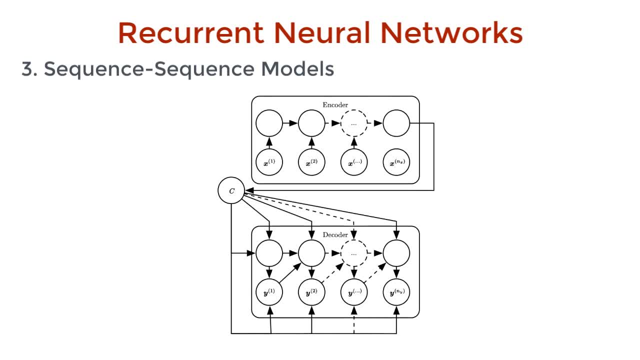 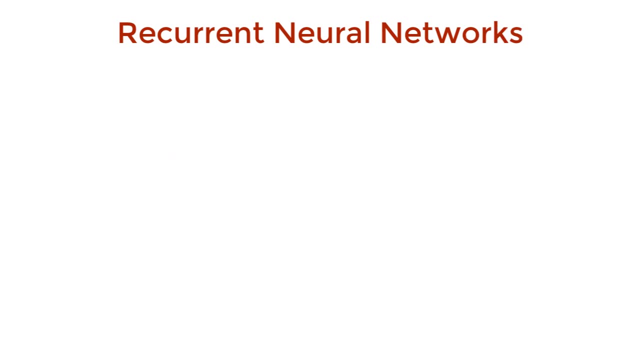 Sequence-to-sequence models is a more popular variant, and these neural networks take in a sequence as input and outputs another sequence. So, for example, language translation: the input could be a sentence in Spanish and the output is the translation in English. Do you have some time? 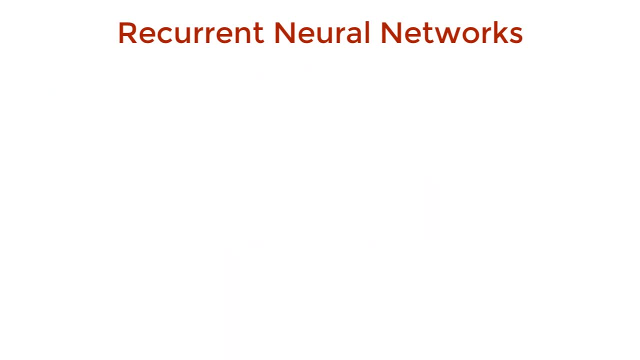 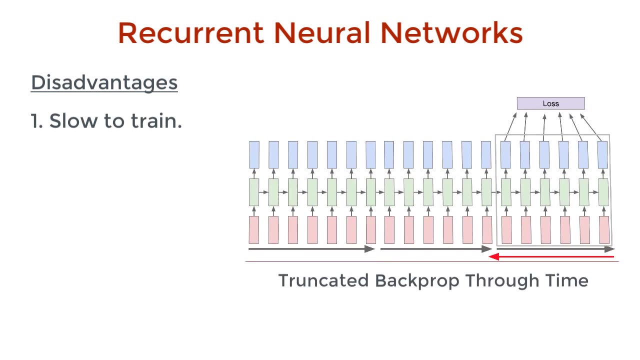 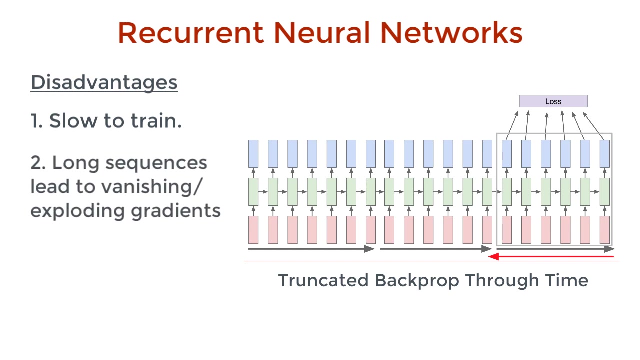 series data to model. Well, RNNs would be the go-to. However, RNNs have some problems. RNNs are slow, So slow that we use a truncated version of backpropagation to train it, and even that's too hardware intense And also they can't deal with long sequences very well. 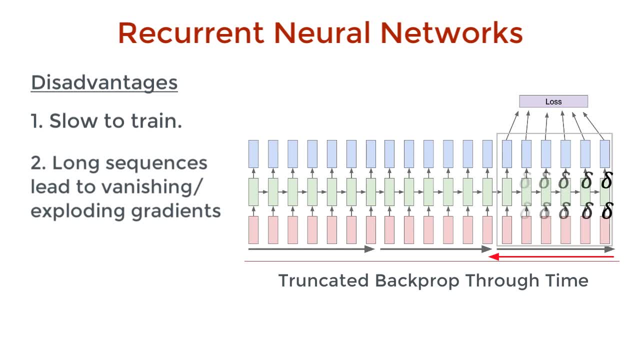 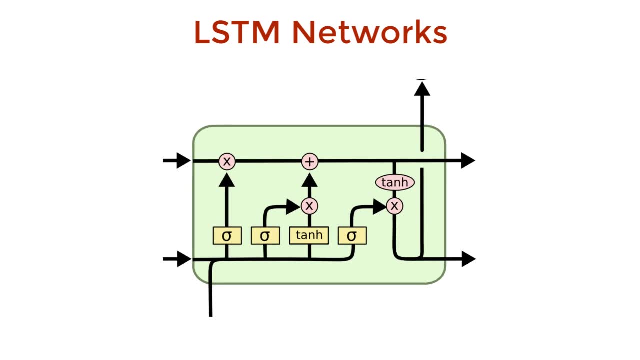 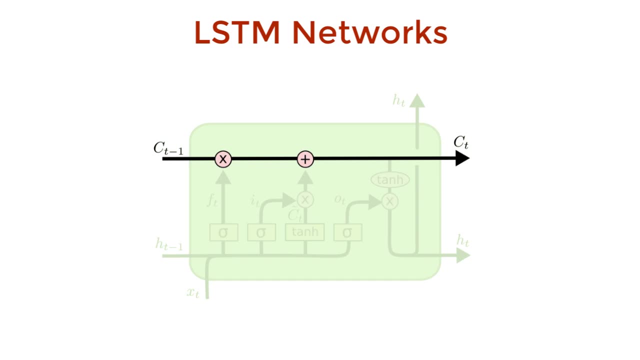 We get gradients that vanish and explode if the network is too long. In comes LSTM networks in 1991 that introduced a long, short-term memory cell in place of dumb neurons. This cell has a branch that allows past information to skip a lot of the processing of. 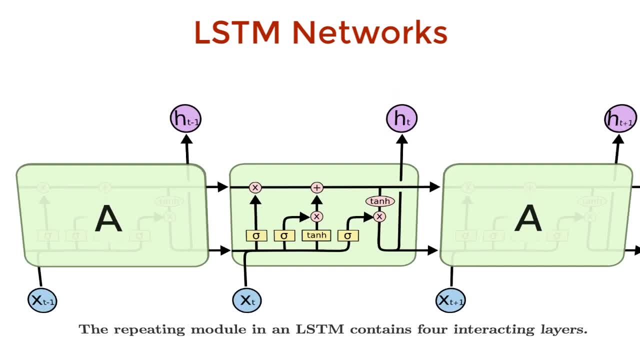 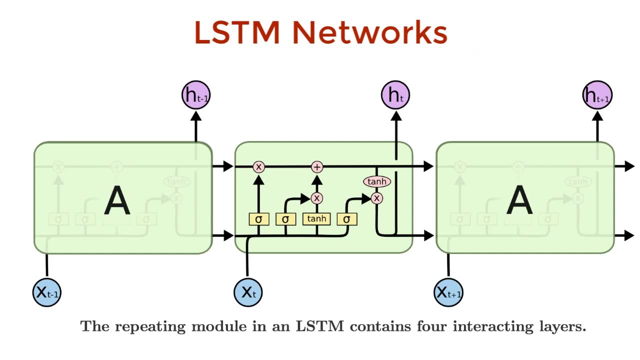 the current cell and move on to the next. This allows the memory to be retained for longer sequences. Now to that second point. we seem to be able to deal with longer sequences well, Or are we Well, kind of Probably, if the order of hundreds of words instead of a thousand. 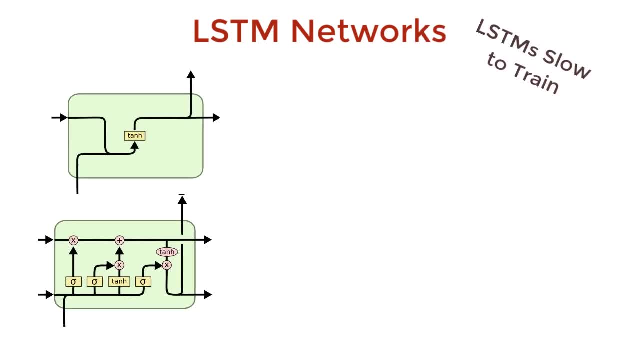 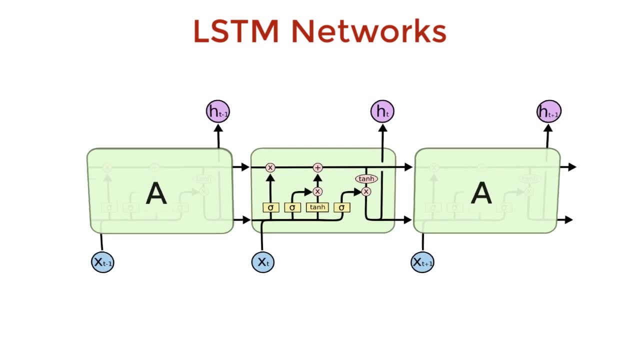 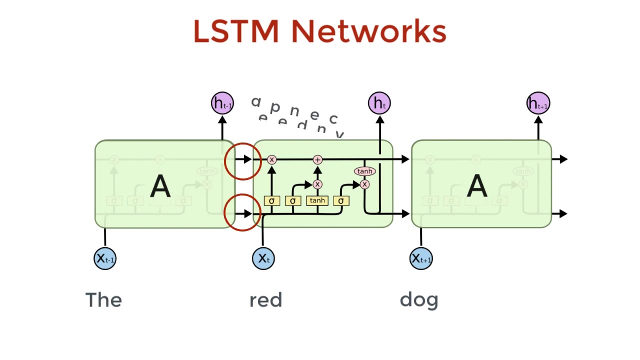 words. However, to the first point. normal RNNs are slow, But LSTMs are even slower. They're more complex. For these RNN and LSTM networks, input data needs to be passed sequentially or serially, One after the other. We need inputs of the previous state to make any operations on the 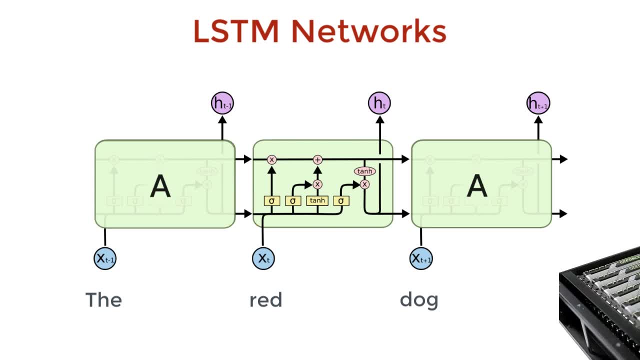 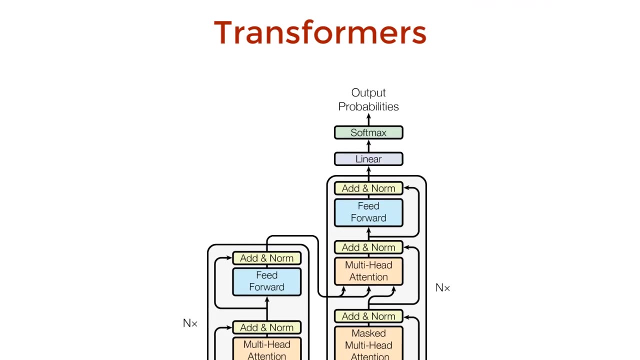 current state, Such sequential flow does not make use of today's GPUs very well, which are designed for parallel computation. So question: how can we use parallelization for sequential data? In 2017, the transformer neural network architecture was introduced. The network employs an encoder-decoder architecture, much like recurrent neural nets. 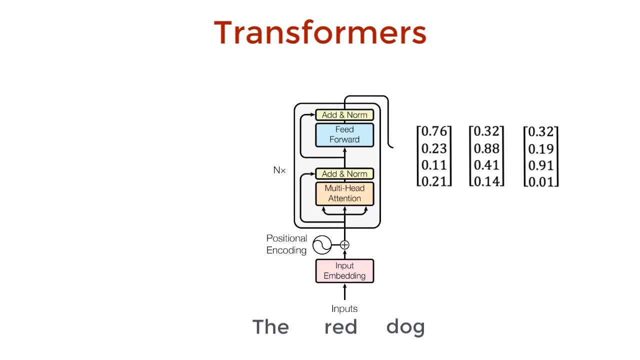 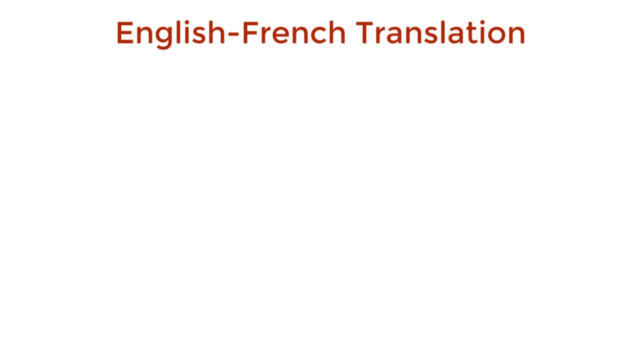 And our jump record demonstrates how The difference is that the input sequence can be passed in parallel. Consider translating a sentence from English to French. I'll use this as a running example. throughout the video, With an RNN encoder, we pass an input English sentence one word after the other. 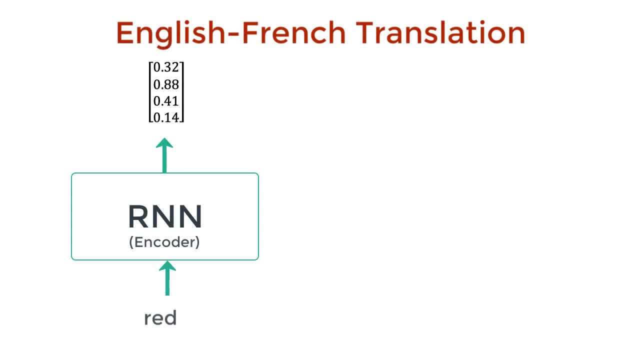 The current word's hidden state has dependencies in the previous word's hidden state. The word embeddings are generated one timestep at time With a transformer encoder. on the other hand, there is no surprising change in the arm synths concept of time step for the input. We pass in all the words of the sentence simultaneously. 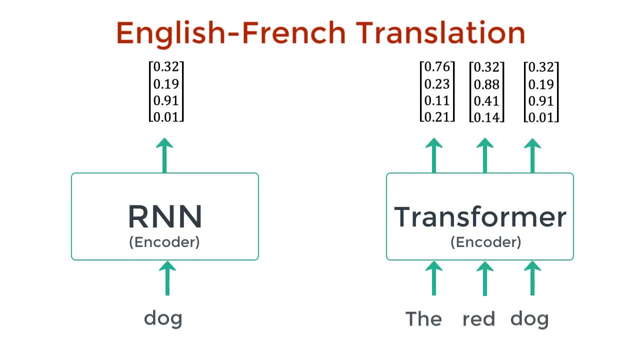 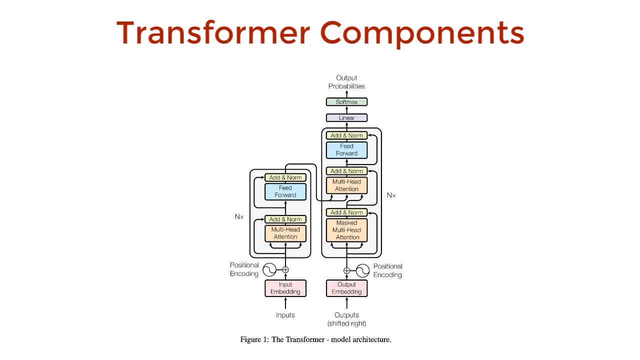 and determine the word embeddings simultaneously. So how is it doing this? Let's pick apart the transformer architecture. I'll make multiple passes on the explanation. First pass will be like a high overview and the next rounds will get into more details. Let's start off with input embeddings. Computers don't understand words, They get numbers. 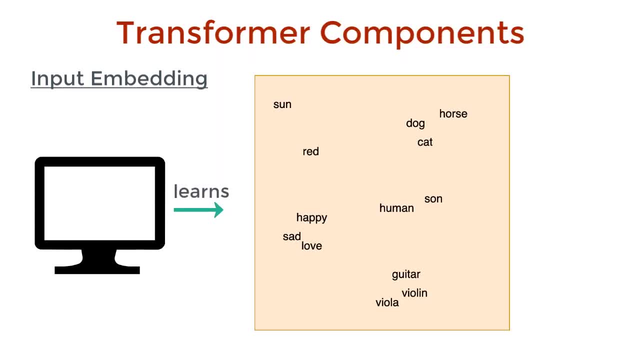 they get vectors and matrices. The idea is to map every word to a point in space where similar words and meaning are physically closer to each other. The space in which they are present is called an embedding space. We could pre-train this embedding space to save time. 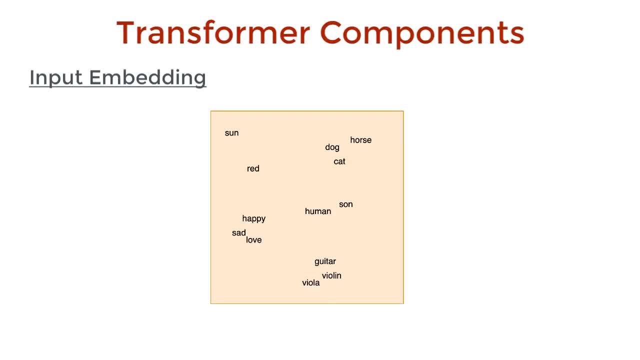 or even just use an already pre-trained embedding space. This embedding space maps a word to a vector, But the same word in different sentences may have different meanings. This is where positional encoders come in. It's a vector that has information that is not properly mapped. It's a vector that has a script that is not. 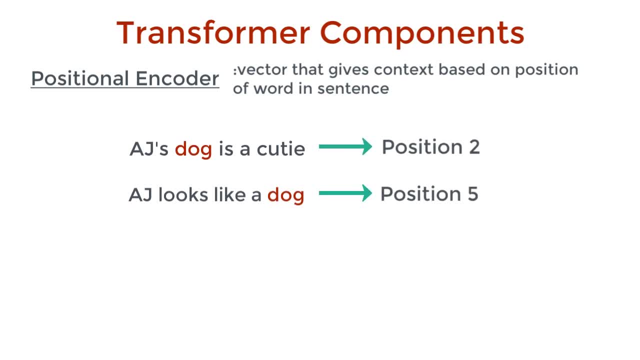 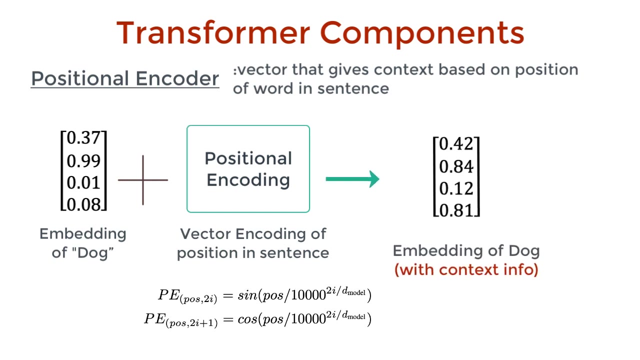 on distances between words in the sentence. The original paper uses a sine and cosine function to generate this vector, but it could be any reasonable function. After passing the English sentence through the input embedding and applying the positional encoding, we get word vectors that have a positional. 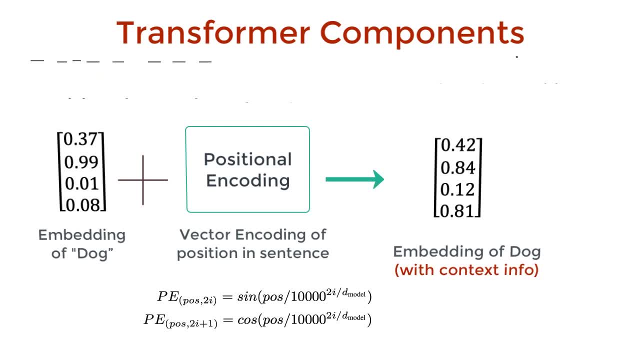 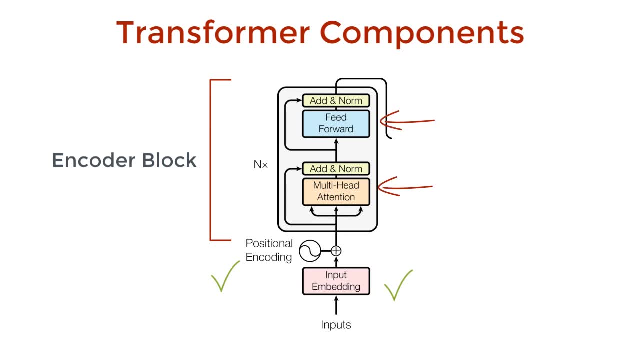 information. that is context. Nice, We pass this into the encoder block where it goes through a multi-headed attention layer and a feed-forward layer. Okay, one at a time. Attention, It involves answering. what part of the input should I focus on If we are translating from English to? 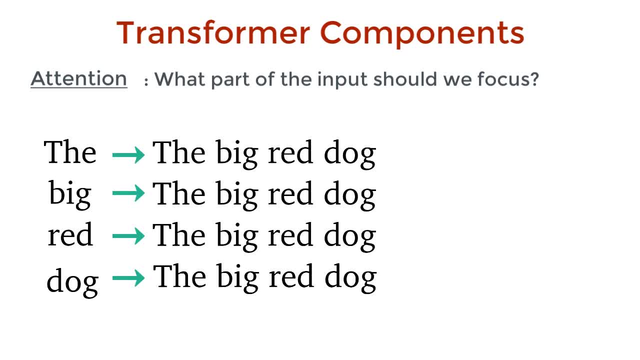 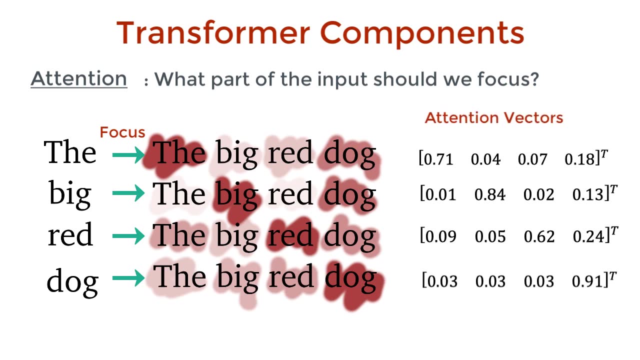 French, and we are doing self-attention, that is, attention with respect to oneself. the question we want to answer is: how relevant is the ith word in the English sentence relevant to other words in the same English sentence? Hmm, Gosh, This is represented in the ith attention vector and it is computed in the attention block. 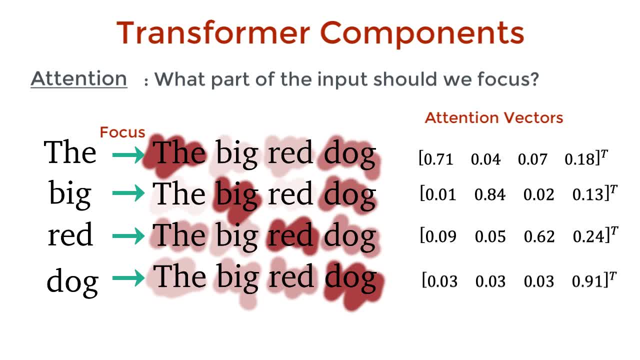 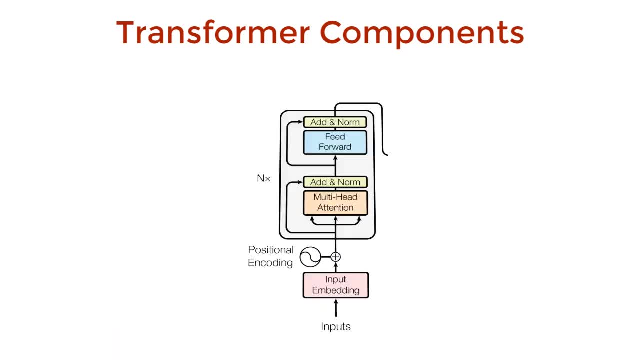 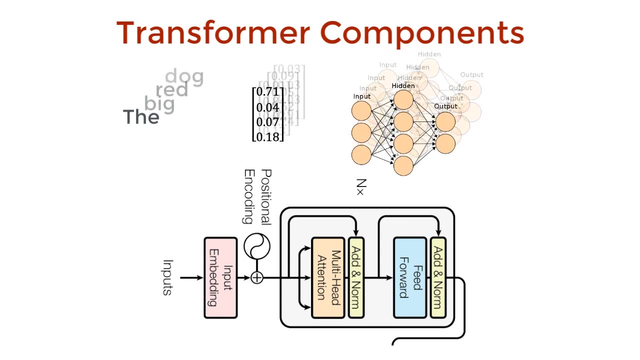 For every word we can have an attention vector generated which captures contextual relationships between words in the sentence. So that's great. The other important unit is a feedforward net. This is just a simple feedforward neural network that is applied to every one of the attention vectors. 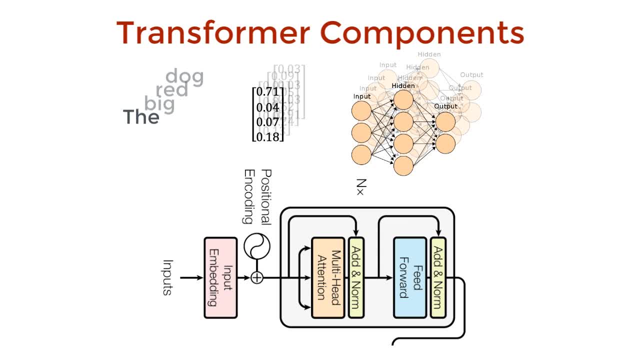 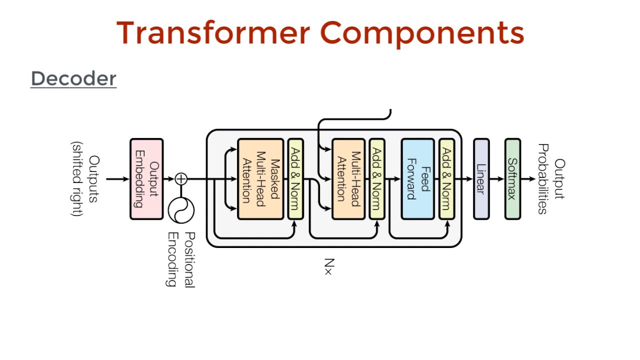 These feedforward nets are used in practice to transform the attention vectors into a form that is digestible by the next encoder block or decoder block. Now, that's the high-level overview of the encoder components. Let's talk about the decoder now. During the training phase for English to French, we feed the output French sentence to the decoder. 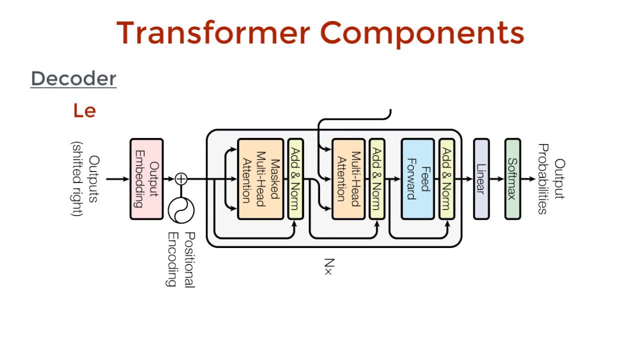 But remember, computers don't get language, They get numbers, vectors and matrices. So we process it. We process it using the input embedding to get the vector form of the word And then we add a positional vector to get the notion of context of the word in a sentence. 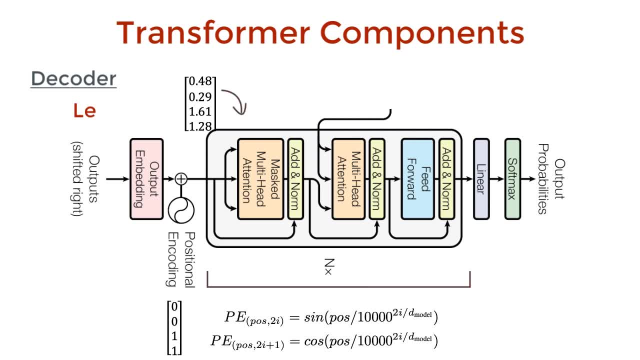 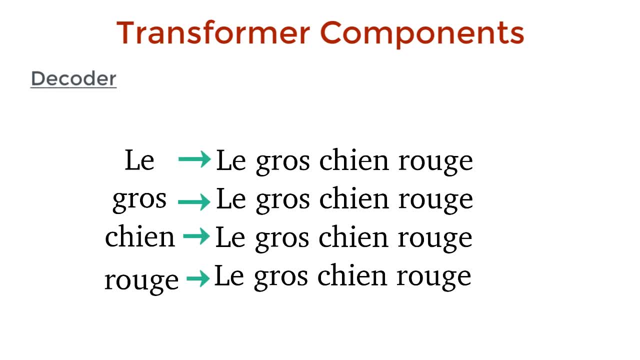 We pass this vector finally into a decoder block that has three main components, two of which are similar to the encoder block. The self-attention block generates attention vectors for every word in the French sentence to represent how much each word is related to every word in the same sentence. 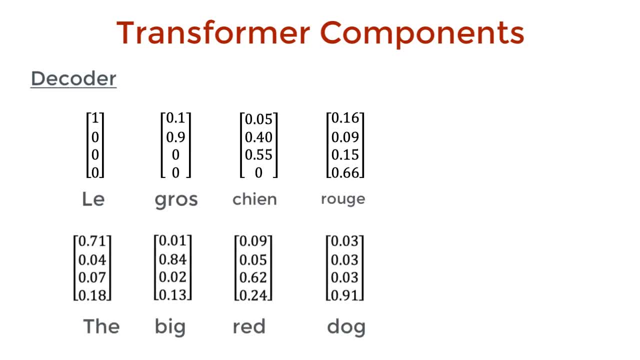 These attention vectors and vectors from the encoder are passed into another attention block. Let's call this the encoder-decoder attention block, since we have one vector from every word in the English and French sentences. This attention block will determine how related each word vector is with respect to each other. 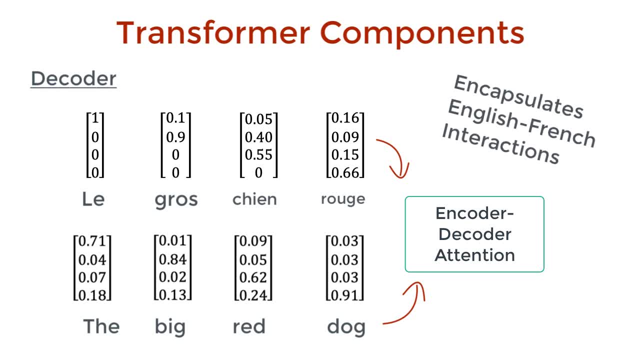 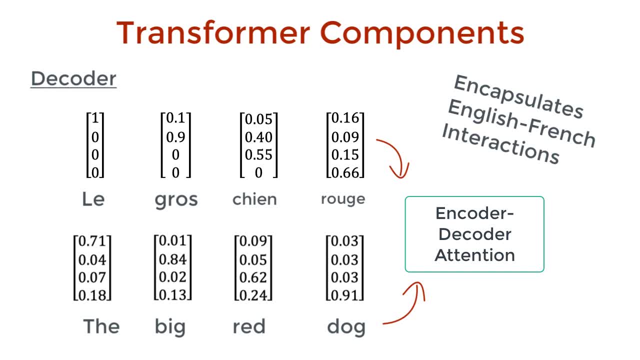 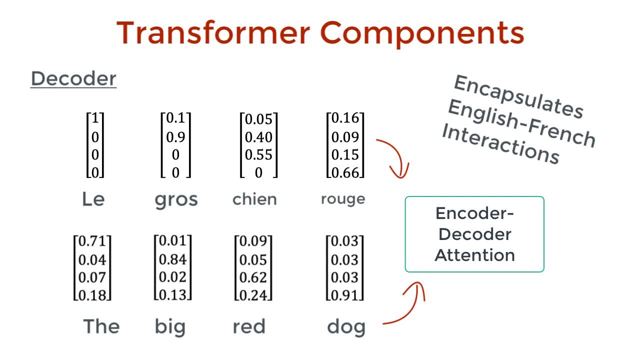 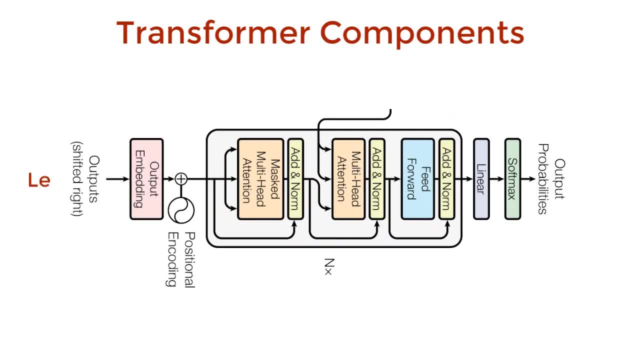 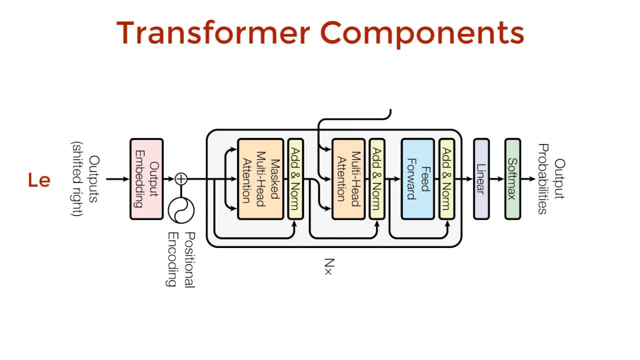 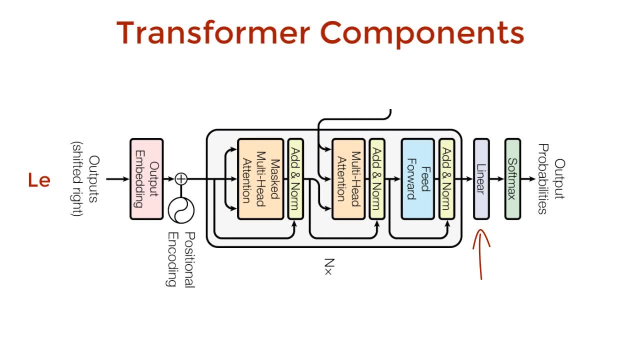 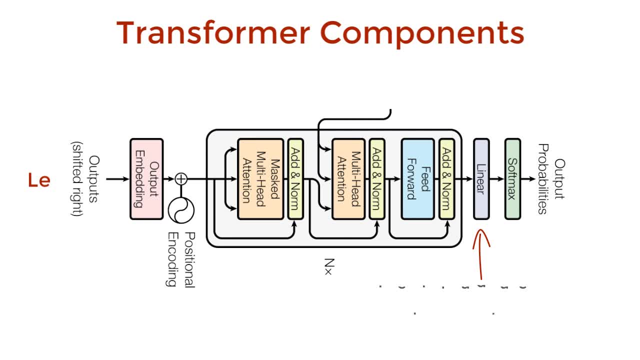 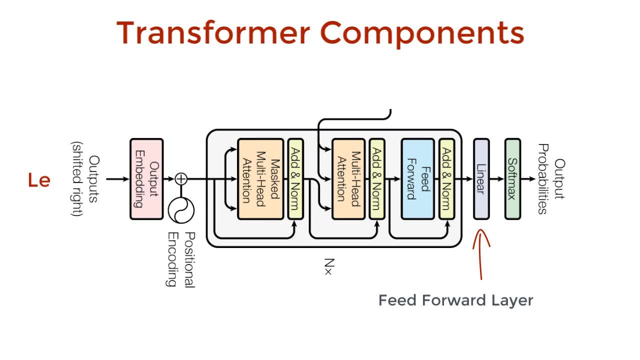 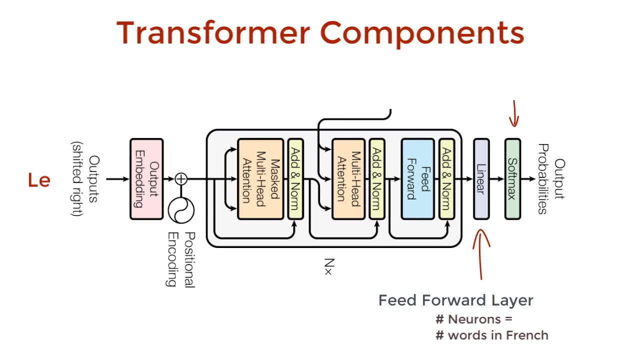 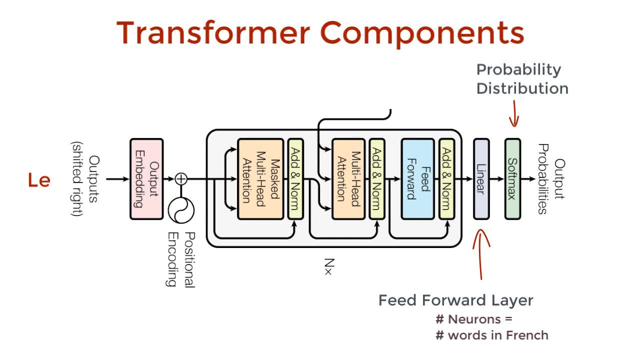 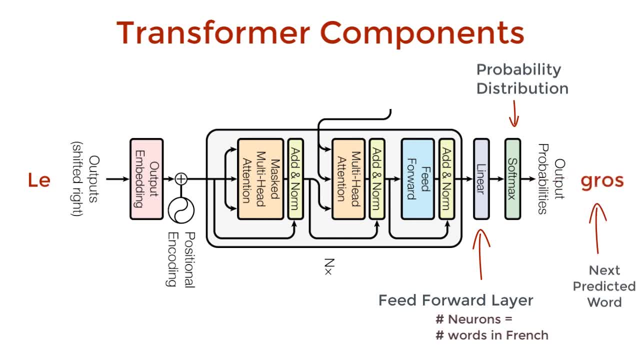 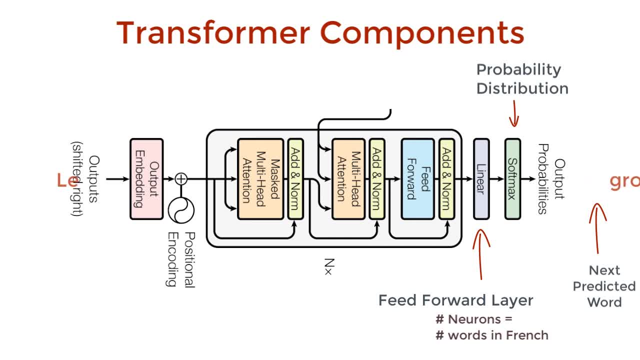 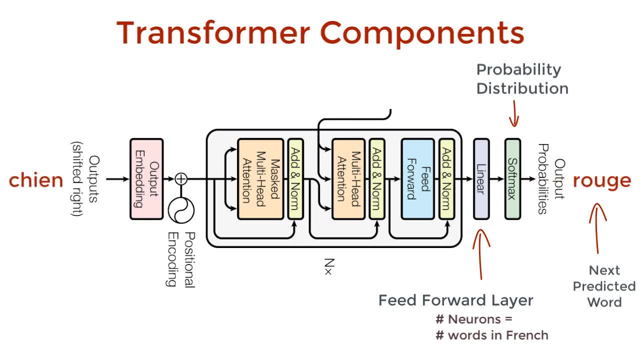 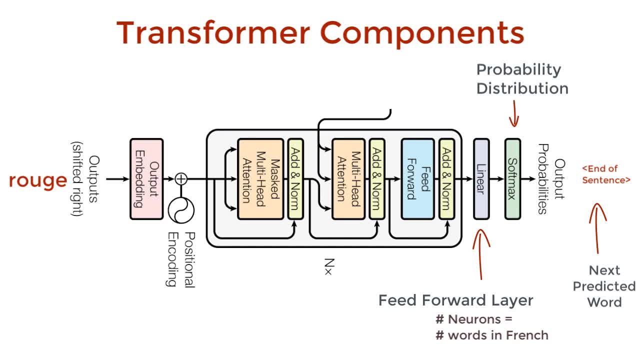 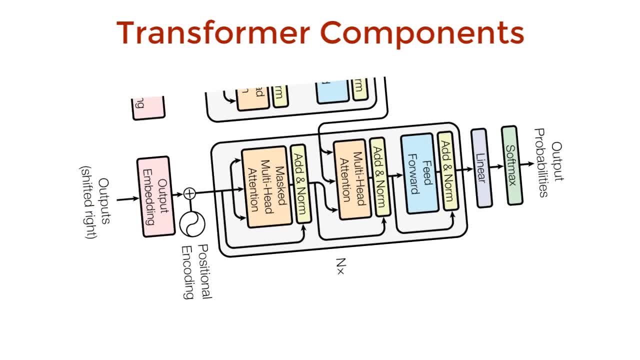 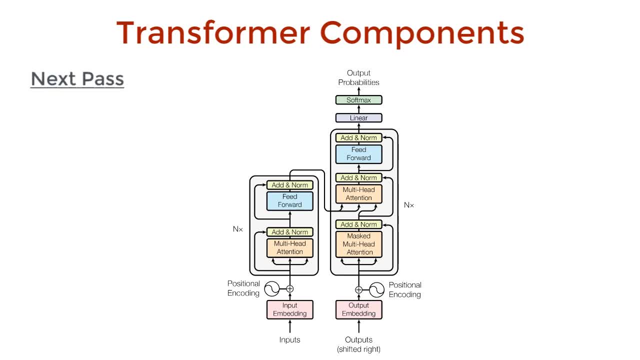 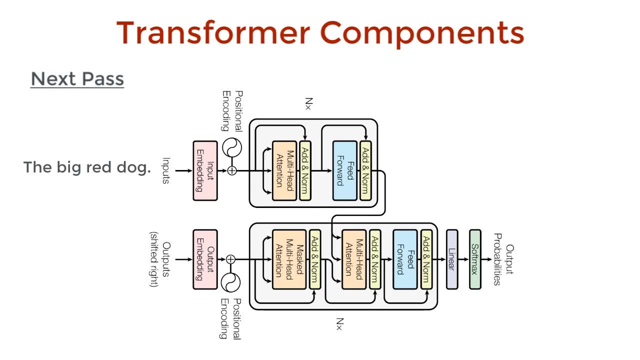 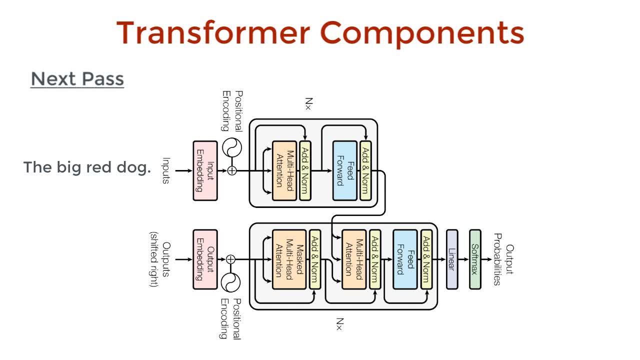 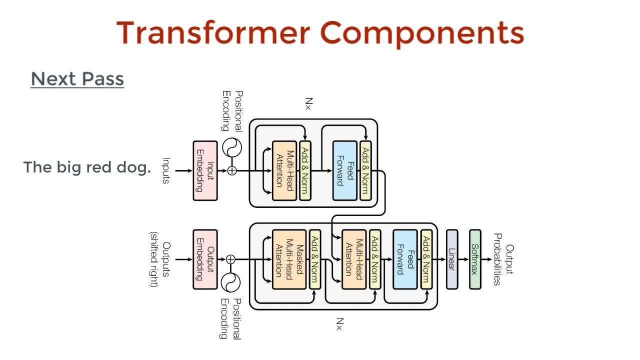 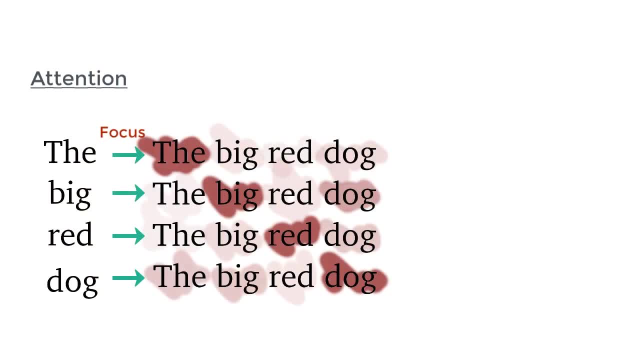 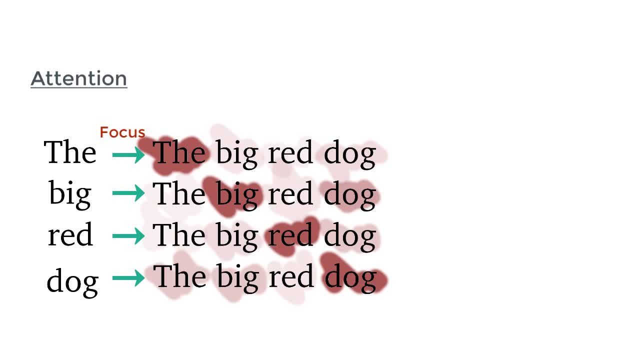 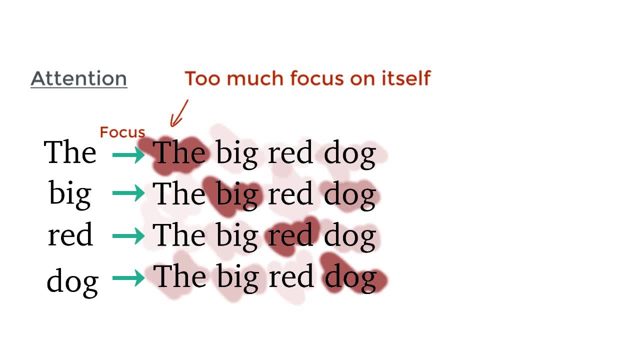 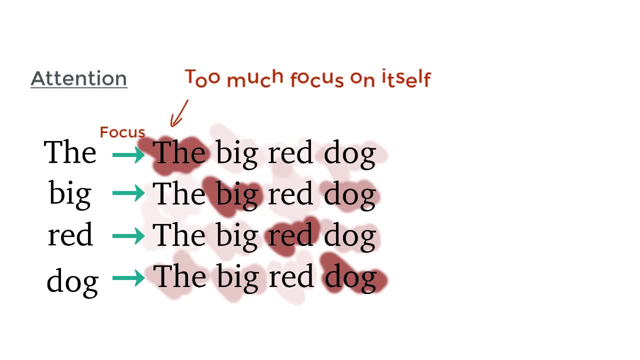 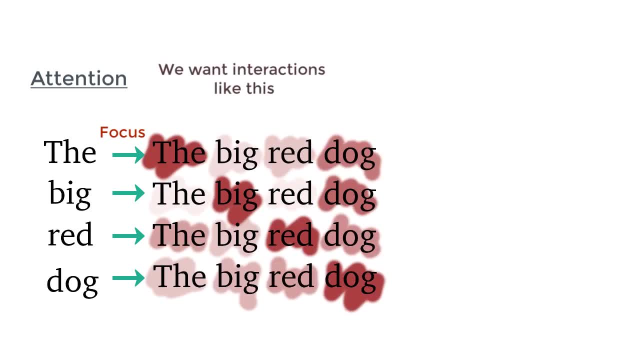 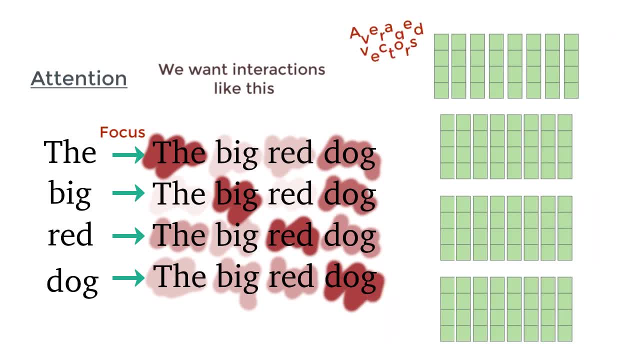 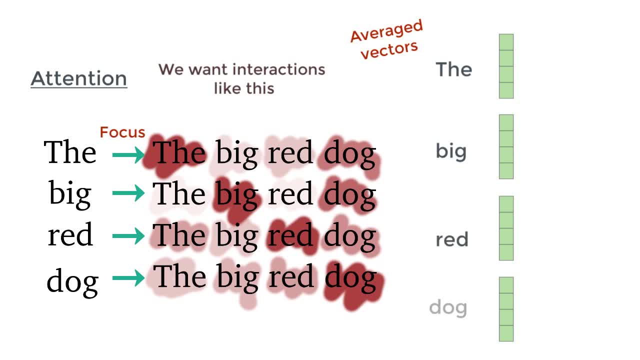 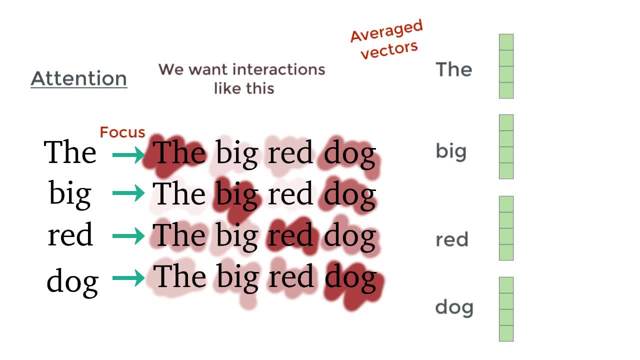 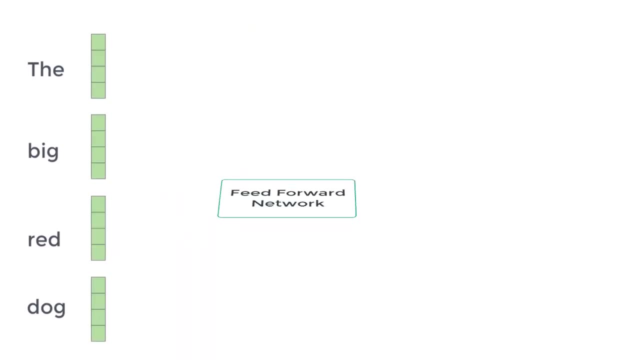 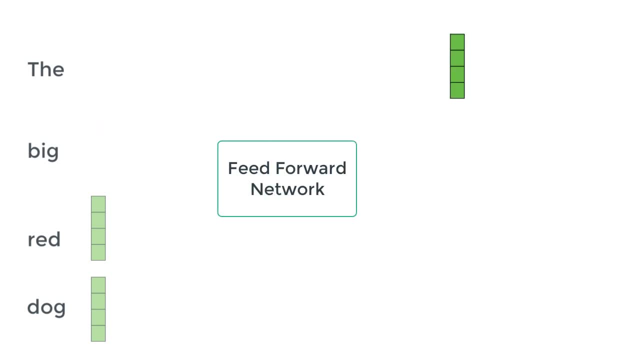 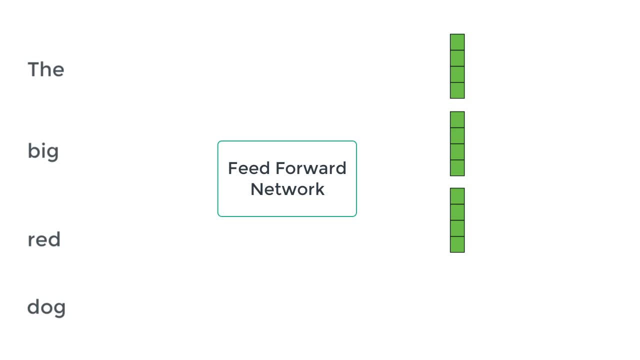 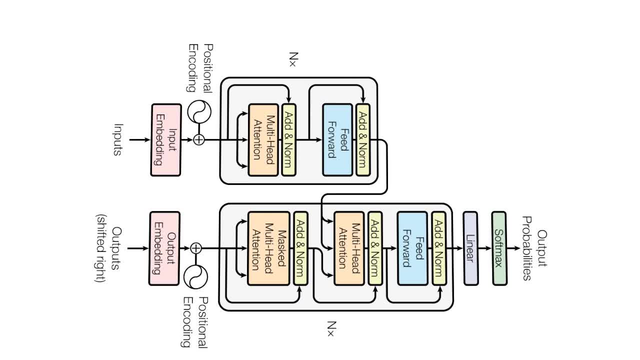 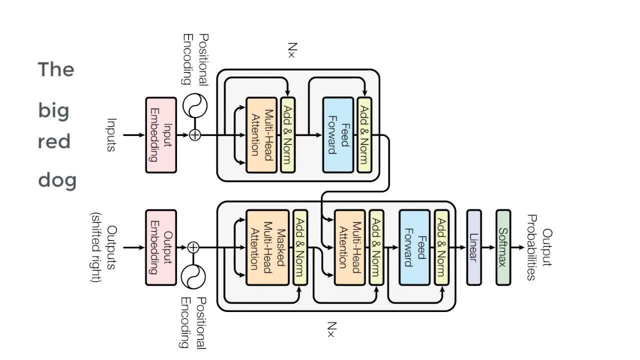 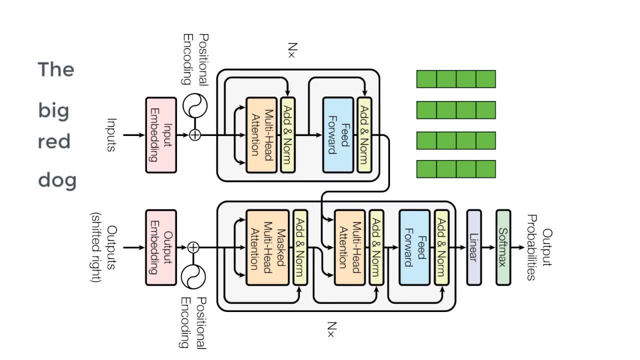 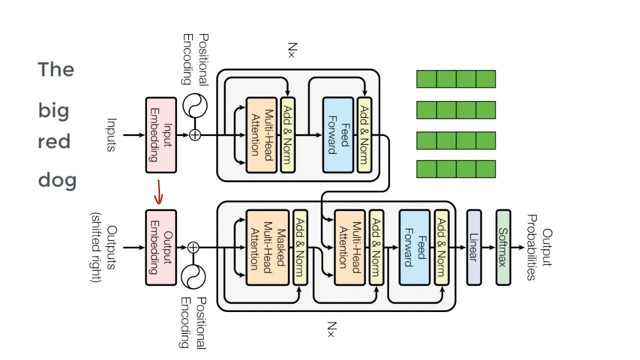 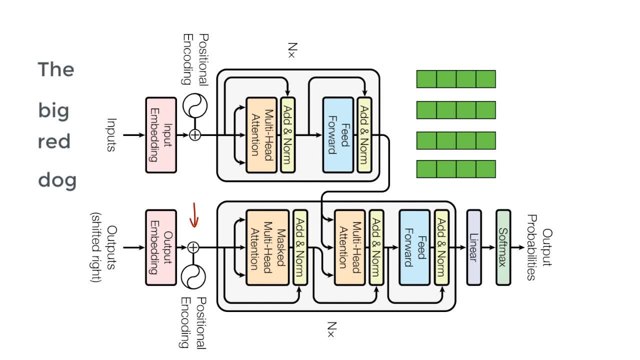 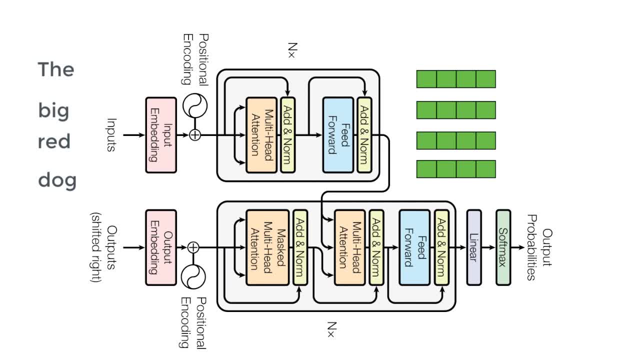 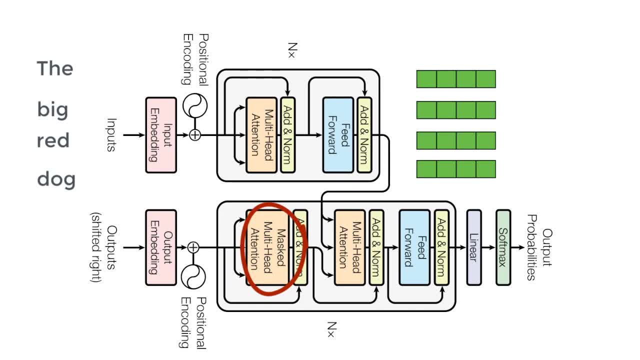 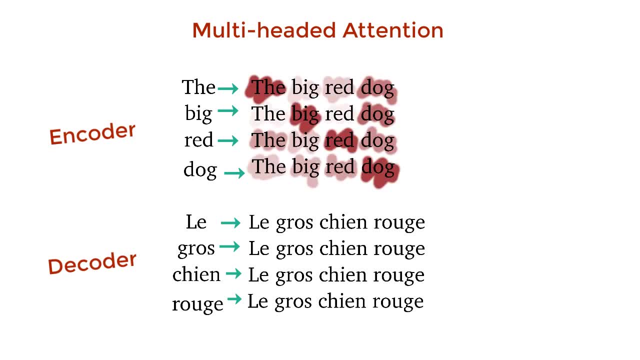 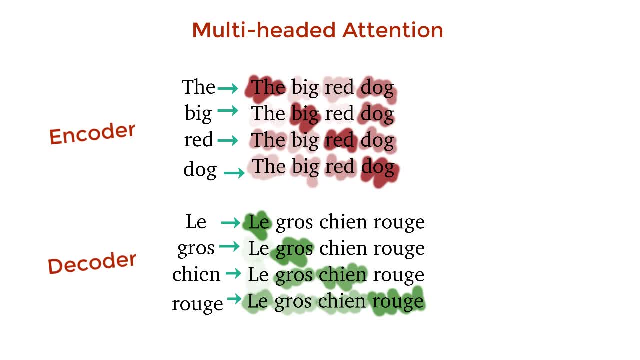 but only the previous words of the French sentence. If we are going to use all the words in the French sentence, then there would be no learning, It would just spit out the next word. So while performing parallelization with matrix operations, we make sure that the matrix will mask. 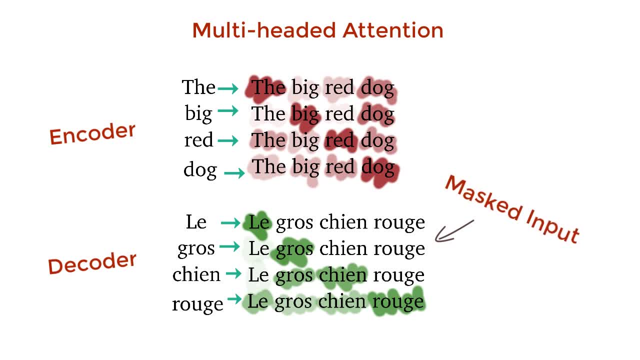 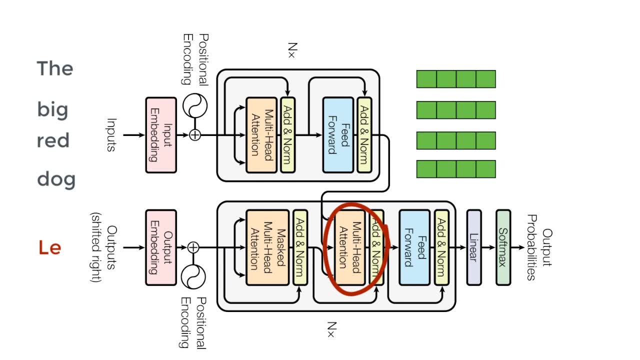 the words appearing later by transforming it into zeros. so the attention network can't use them. The next attention block, which is the encoder-decoder-attention block, generates similar attention vectors for every English and French word. These are passed into the feed-forward layer. 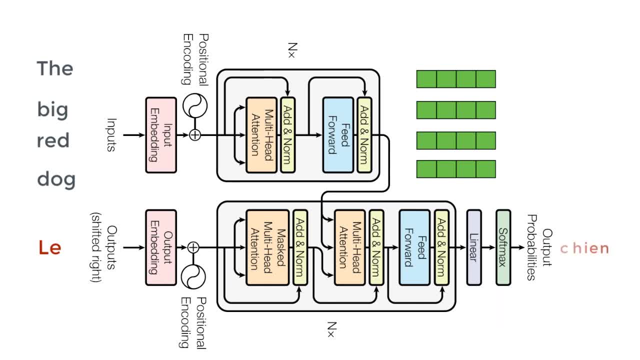 linear layer and the softmax layer. to predict the next word, That's the past two- over the architecture. explain, I hope you're understanding more and more details here. Now for the next part. we're gonna talk about the multi-head attention networks. 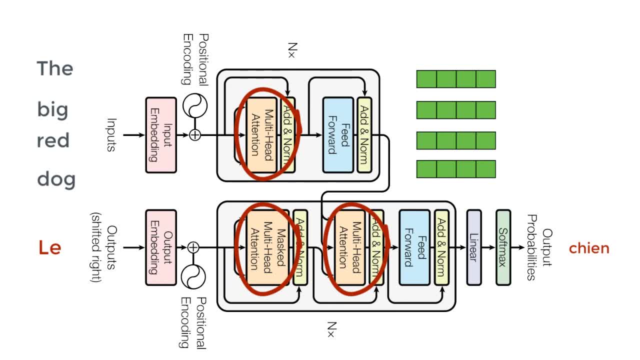 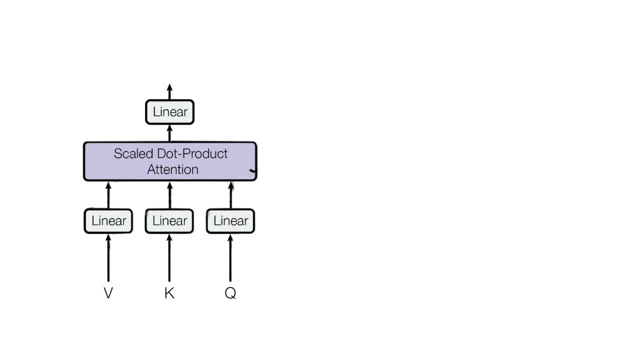 How exactly do these multi-head attention networks look? Now the single-headed attention looks like this: Q, K and V are abstract vectors that extract different components of an input word. We have Q, K and V vectors for every single word. 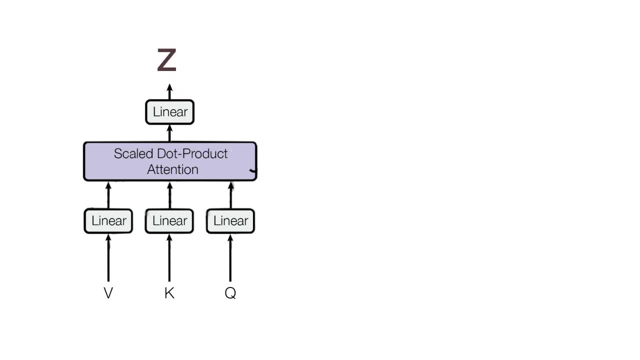 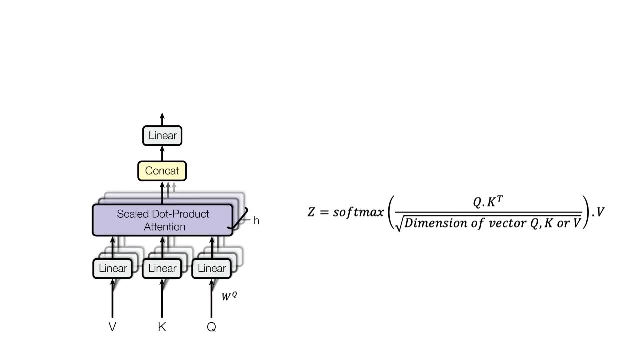 We use these to compute the attention vectors for every word, using this kind of formula. For multi-headed attention. we have a formula attention. we have multiple weight matrices- wq, wk and wv- so we will have multiple attention vectors- z- for every word. however, our neural net is only expecting one attention vector per word. 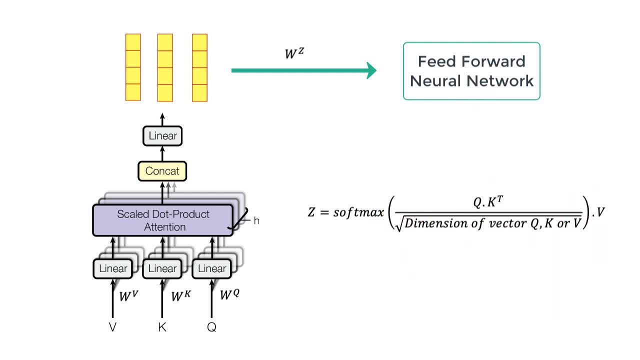 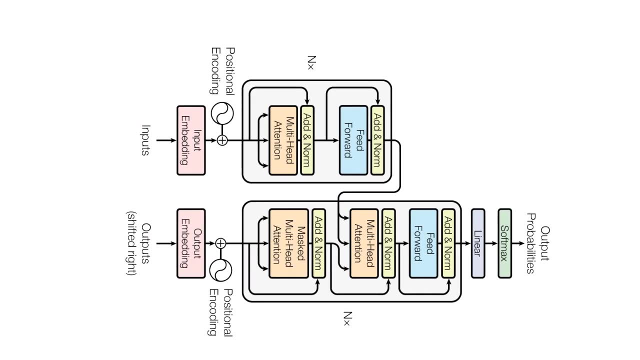 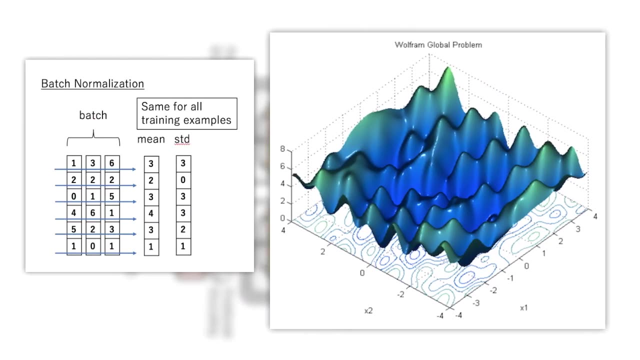 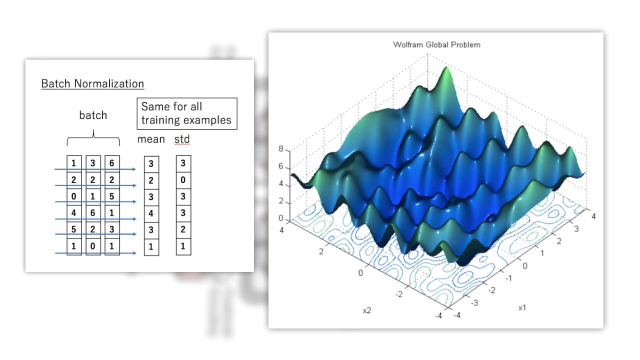 so we use another weighted matrix, wz, to make sure that the output is still an attention vector per word. additionally, after every layer, we apply some form of normalization. typically we would apply a batch normalization. this smoothens out the lost surface, making it easier to optimize while using larger learning rates. this is the tldr, but that's what it does, but we can actually use. 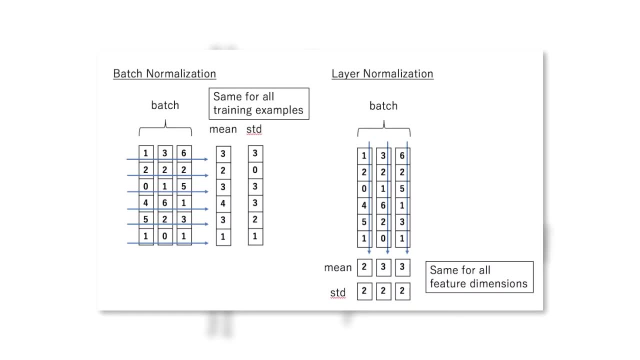 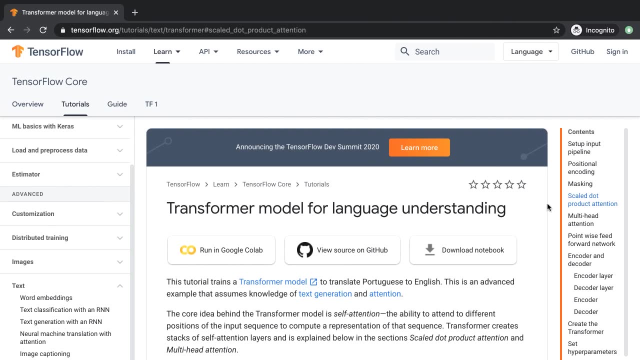 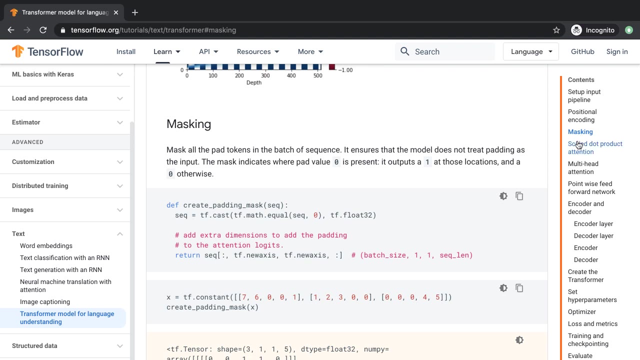 something called layer normalization, making the normalization across each feature instead of each sample. it's better for stabilization. if you are interested in dabbling in transformer code, tensorflow has a step-by-step tutorial that can get you up to speed. transformer neural nets have largely replaced lstm nets. for sequence to: 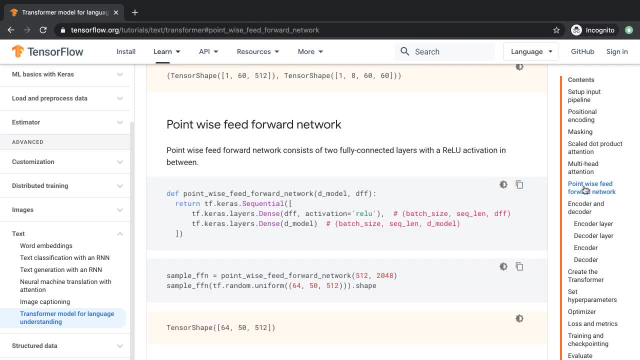 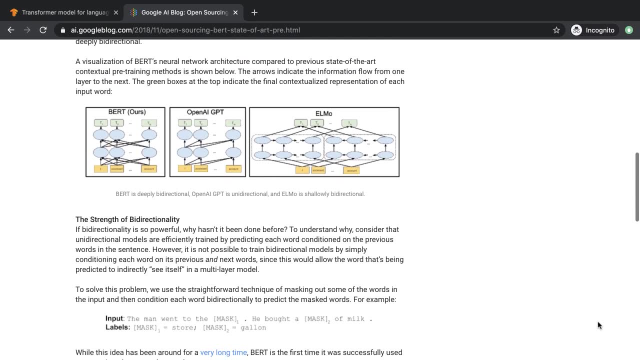 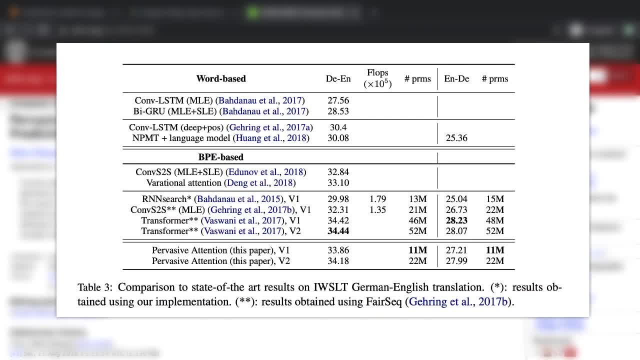 go over it and we're going to take a look at it and we're going to take a look at it and we're going. better than transformers for sequence to sequence models, although transformers can be better suited for a wider variety of problems. it's still a very interesting read. i'll link it in the description. 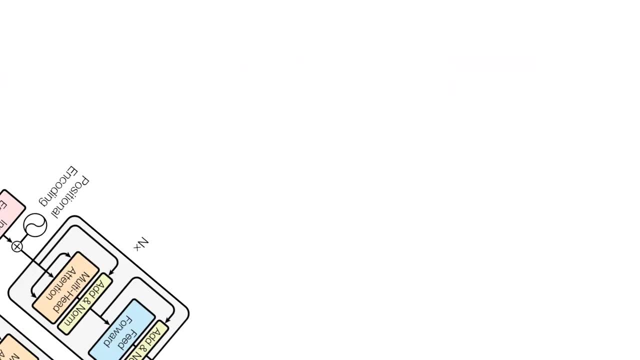 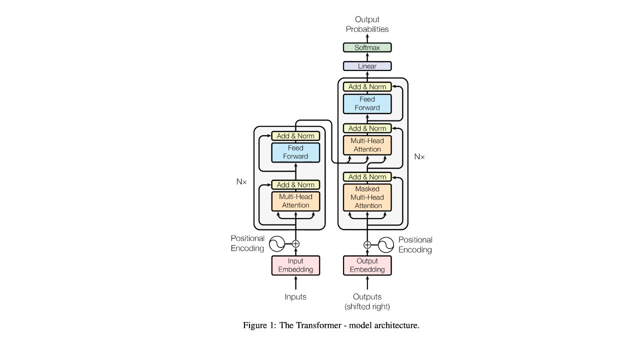 below with other resources, so check that out. hope this helped you get you up to speed with transformer neural nets. if you liked the video, hit that like button- subscribe- to stay up to date with some deep learning and machine learning knowledge, and i will see you guys in the next one. bye you.